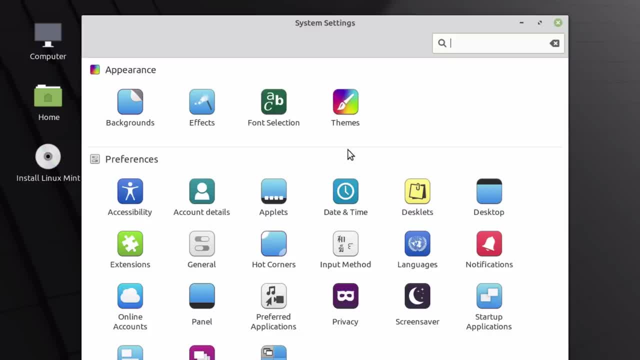 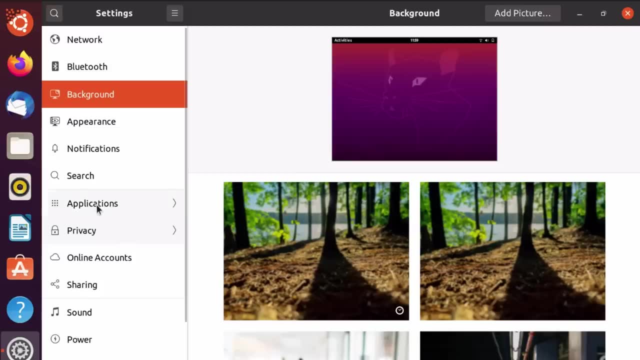 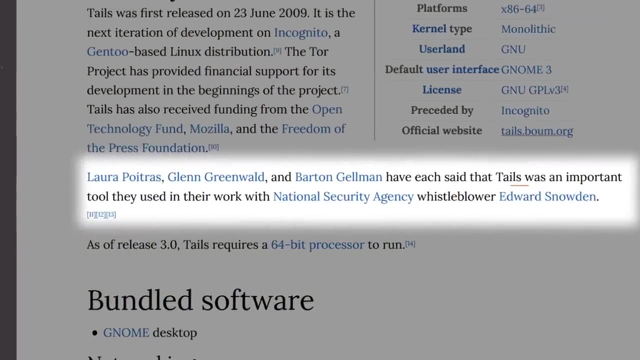 agencies. Then there are common Linux distributions like Mint, Debian and Ubuntu. These are all a big step in a more private and secure direction, but these weren't the ones Snowden recommended Back in 2013,. Snowden in fact used the operating system Tails to communicate with journalists. 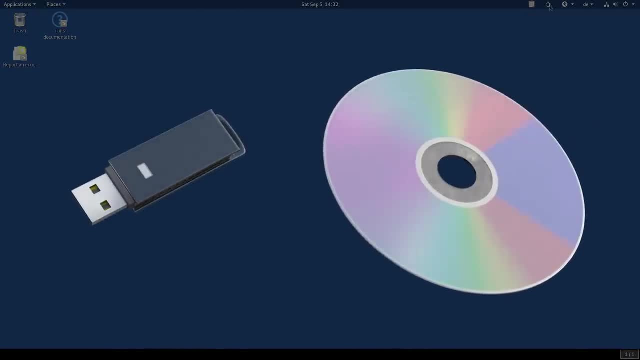 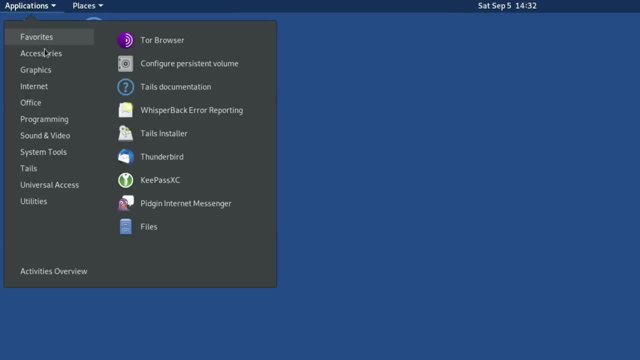 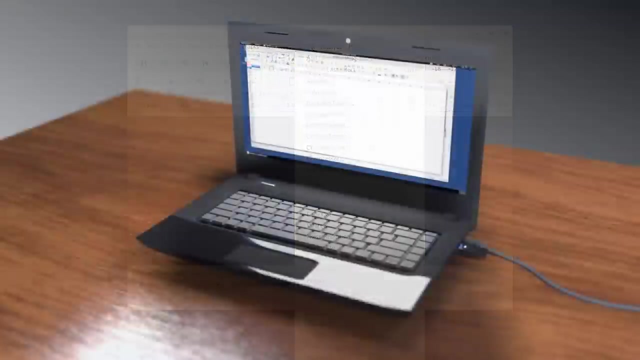 It is designed to be booted as a live DVD or USB and to leave no trace on the machine. This already hints at the fact that it is not intended to replace a fully-featured everyday operating system, but rather for specific sensitive tasks. The advantage is you can even use it on other people's computers and carry selected documents. 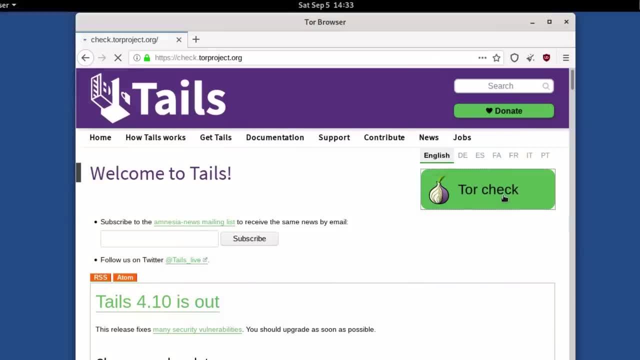 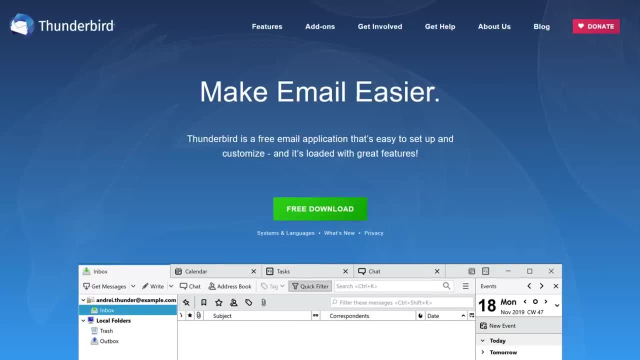 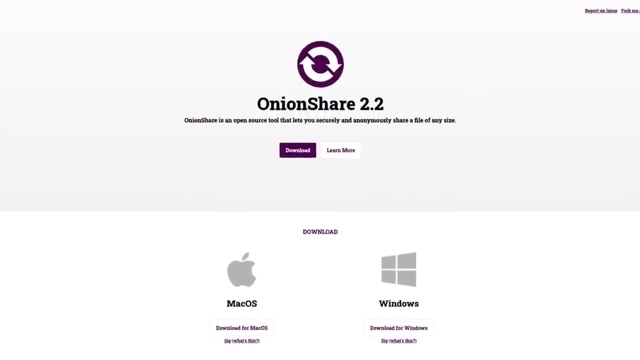 and settings in an encrypted persistent storage of Tails. All network traffic is automatically routed through the Tor network for anonymous communication, and Tails includes some useful tools like an email client, a password manager, an office suite and a file-sharing application. Tails helps to avoid online surveillance, censorship and tracking and is one of the 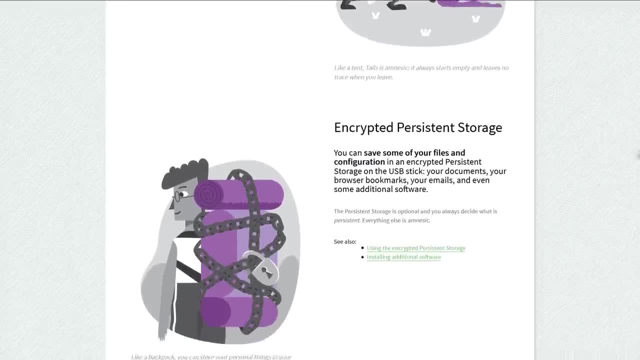 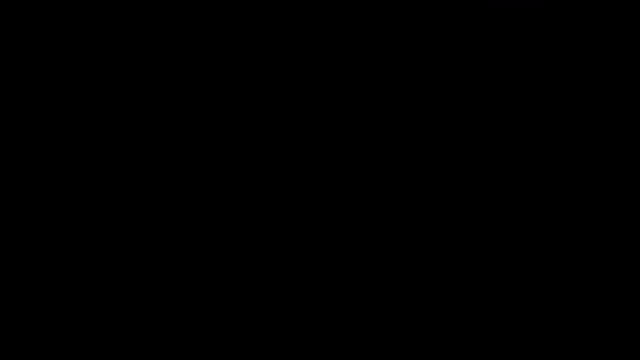 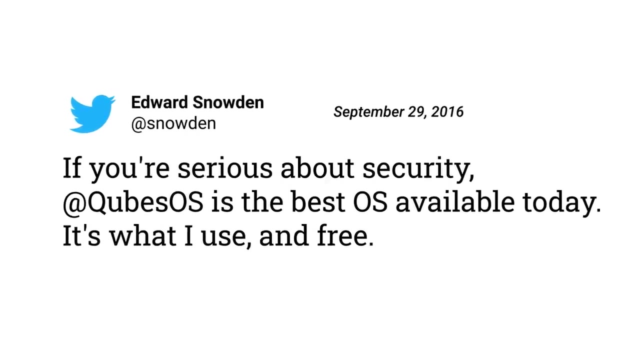 few operating systems that aren't even easily compromised by physical access. because of its temporary nature, Everything the user did disappears once it's shut down. A few years later, in 2016,, Edward Snowden recommended another operating system. Seemingly he had replaced Tails. 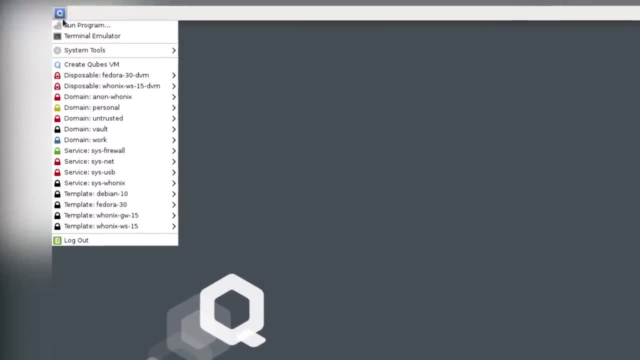 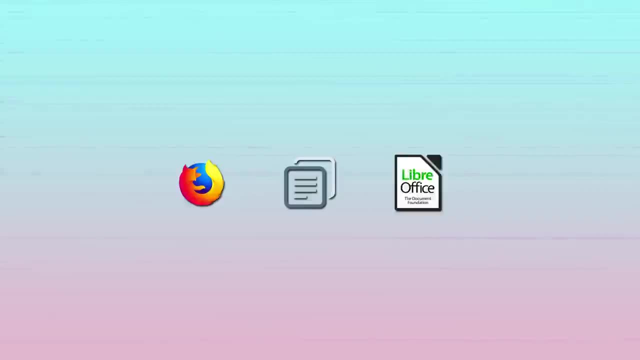 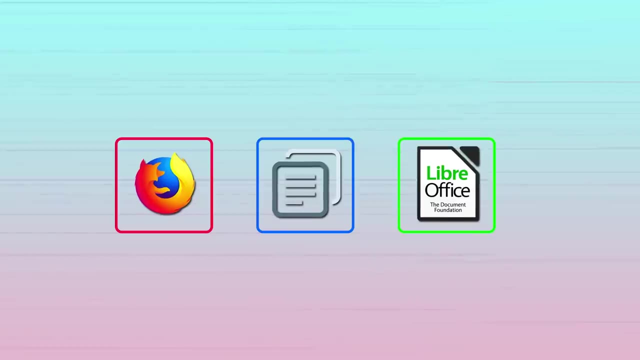 He tweeted about Cubes OS, a system that is all about security by isolation. Contrary to Tails, it can be used as a permanent operating system. Cubes uses virtualization technology to isolate various programs from each other and even sandboxes many system components, like networking and storage. 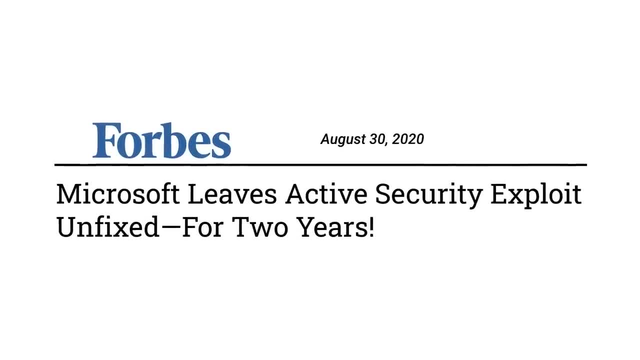 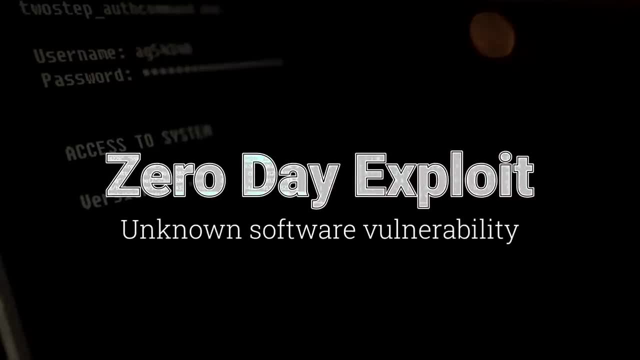 This way, even if one of these programs or components is vulnerable to attacks, it does not affect the integrity of the entire system. It's one of the most effective ways to keep the system safe. It's one of the most effective ways to defend against zero-day exploits. 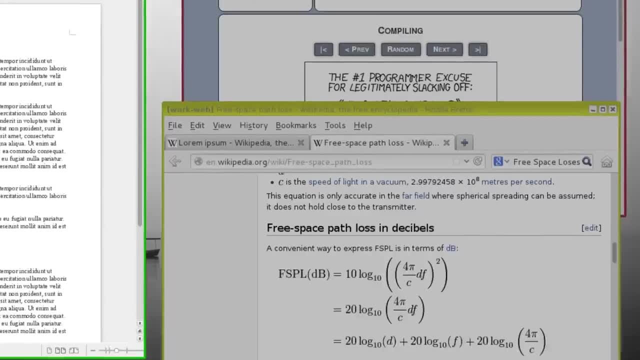 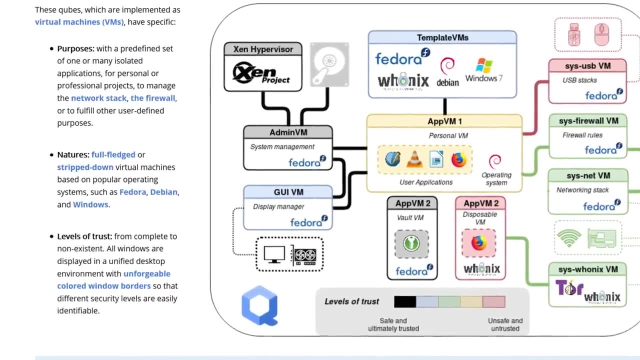 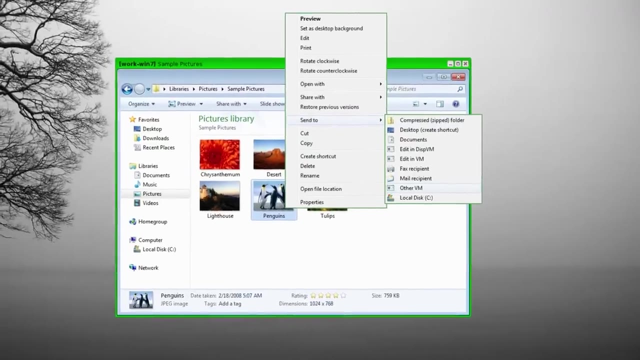 Every window in Cubes has a certain color to indicate in which domain it runs, fully isolated from other domains. The isolated compartments called Cubes, like the operating system, are categorized by purposes, level of trust and template. virtual machines. Apart from popular Linux distributions like Fedora and Debian, Cubes can also run Windows.